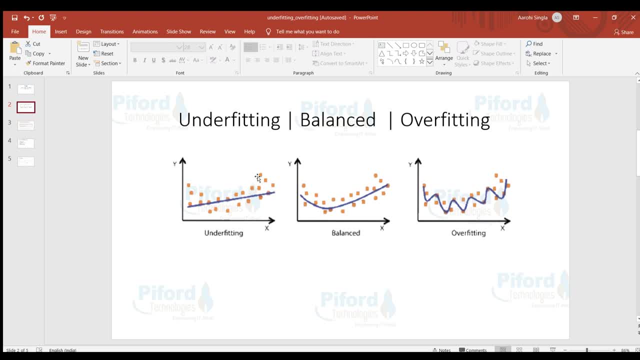 is showing the prediction of our algorithm, So most of the data points are away from this line. That simply means the algorithm which we are applying on this particular data set. that algorithm is not able to learn properly this data, So I'll explain you in detail what is underfitting and how we can. 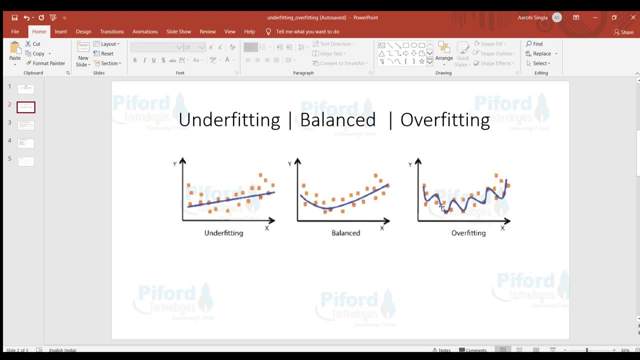 reduce it. But first of all let's understand the basic terms meaning. So underfitting simply means model is performing poor on training data. Model is not able to learn this particular data right. So this is the balanced, you know balanced thing. Balance simply means that this is how your 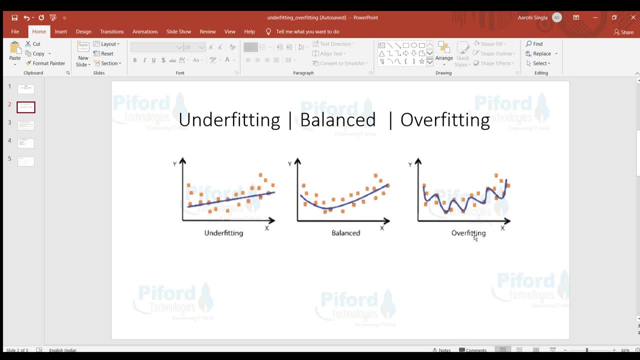 algorithm should work right And what is underfitting So underfitting is the algorithm is overfitting. Over here you'll see that model is performing too good means 100% accuracy is there right? Means as our data. the same way our data is moving, algorithm is also predicting the 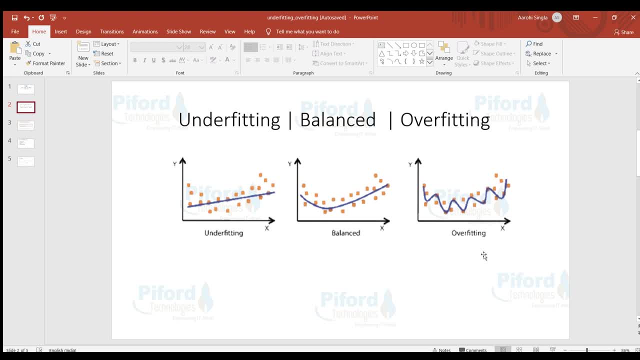 same way. So this is again a big problem, because overfitting simply means when your algorithm is working well on training data, but at the time of testing your algorithm is not performing well. Means, While training it is performing well, but while testing your algorithm it is not performing well. 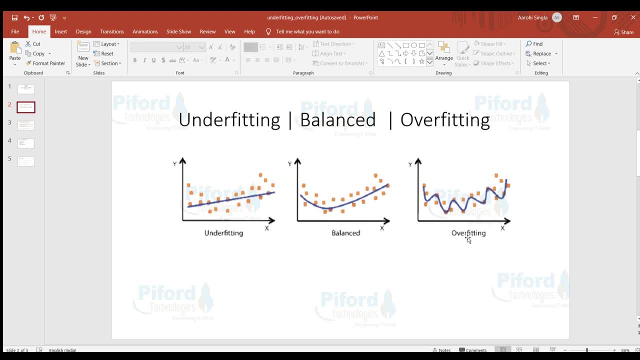 So now we will discuss each of these terms one by one. So let's start with overfitting. So what I've explained you in overfitting, that model performed well on training data, but it is not performing well on test data. So how you can check that? So this is how we check the accuracy. 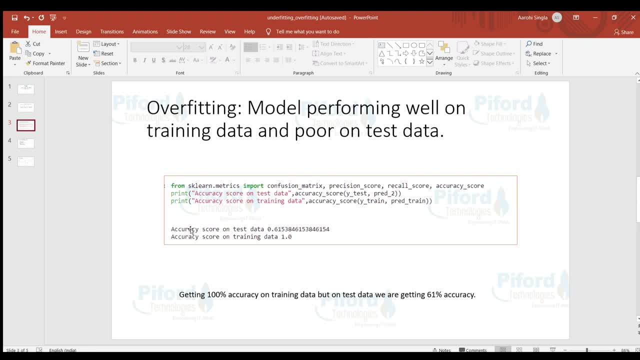 right. So over here, if you'll see, accuracy score on test data is 61%, But the accuracy score on training data is 100%. means model is performing well on training data. on training data It is giving us 100% accuracy, but on test data it is only giving us 60% accuracy. 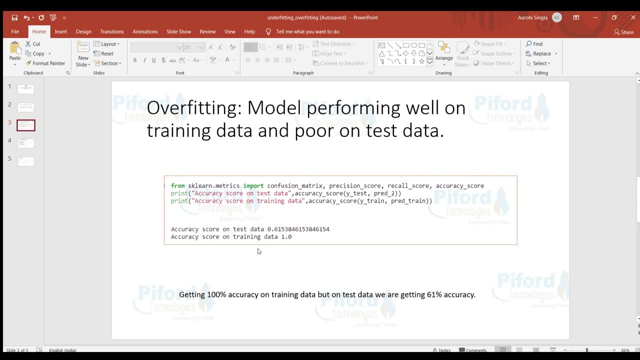 So that means here is a problem of overfitting. and what overfitting is exactly? overfitting simply means That your algorithm is Remember the things instead of learning, means your algorithm is not learning right what it what it is doing. it is only memorizing the things right. and if your algorithm is overfitting the 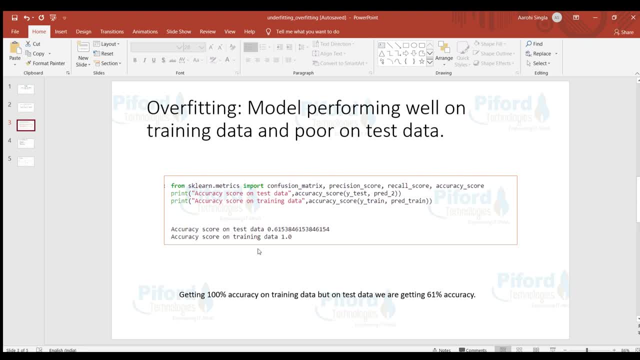 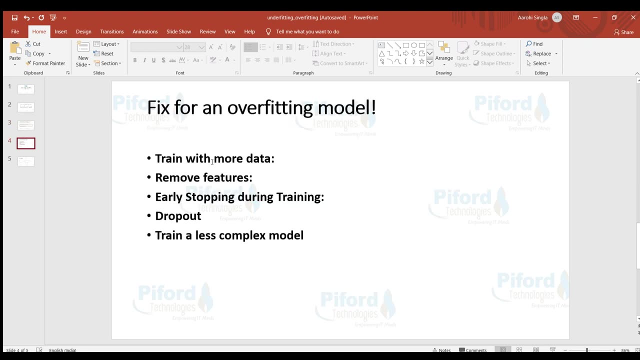 training data, then how we can, you know, solve this problem. now the challenge is: if overfitting is there in your algorithm, then how we can reduce the problem, how we can solve this problem. so how we can solve this problem. so these are the few ways by which we can solve the problem. 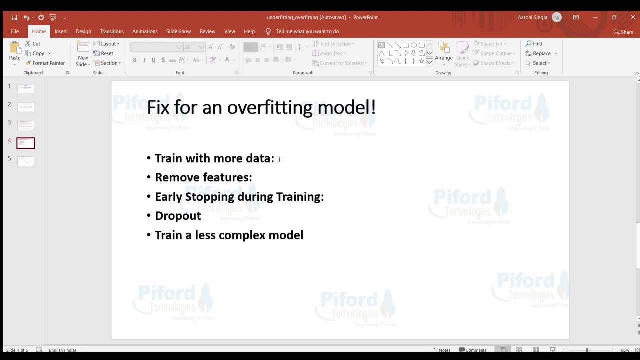 the very first thing is: train with more data means increase your data, right, so increasing the training data, you can even use data augmentation for it. so if you have heard about data augmentation, that simply means increase your data and how we can increase data by using data augmentation techniques- data, 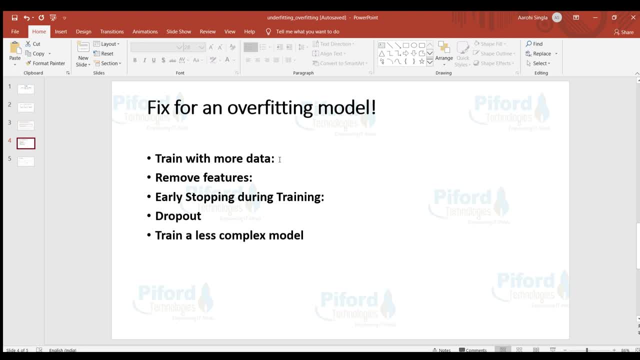 augmentation simply means it will generate more data from the current available data. so you can use data augmentation techniques or you can use other ways to increase your data, because when your algorithm will be having more data, then it will try to learn instead of memorizing the things. 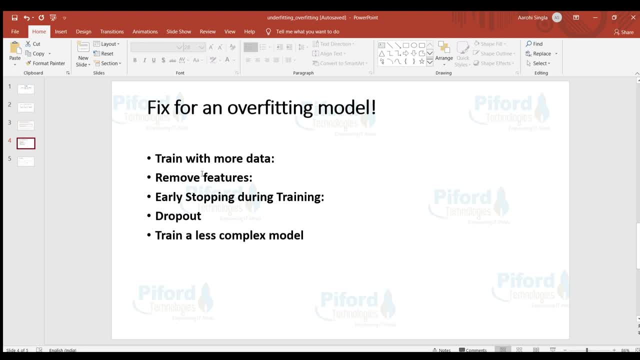 right. and the second thing is remove features. see, we all have studied about feature selection in machine learning, right? so what is feature selection? feature selection means simply change the data from the current available data so you can use data augmentation techniques, choose the best features, on the basis of which your algorithm will give you good results, means: 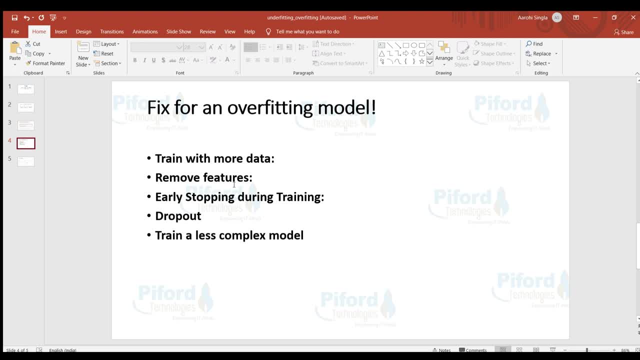 delete all the useless features. and, after removing all those useless or unnecessary features, try to train your algorithm right. and the third thing is early stopping during training. so this step, if you want to perform this early stopping, this can be done in deep learning only. so what this early stopping is? early stopping simply means that you can use data augmentation techniques to 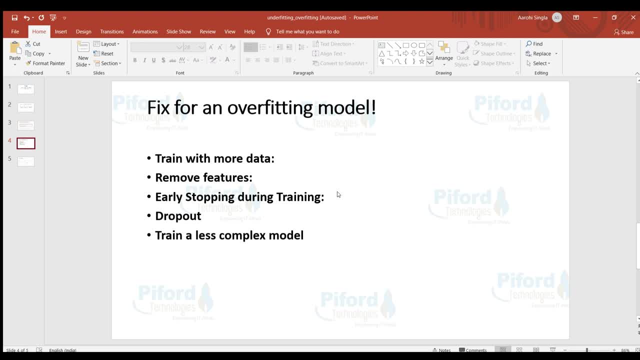 improve the results. you can. you know what you do is. you can use this in deep learning and when you have higher number of epochs, then you can use early stopping. when your model stop- you know improving the results- and it start- you know overfitting- then you can use early stopping. 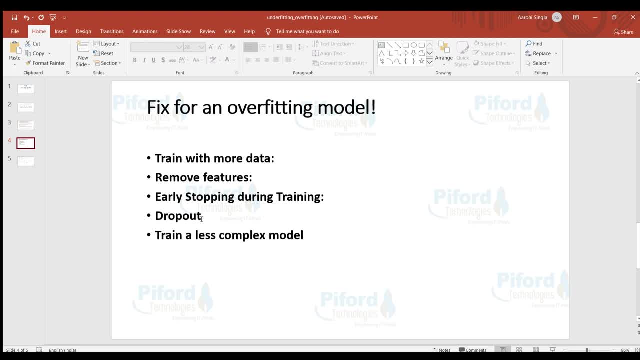 to stop the training process, and then the next is dropout. see, dropout simply means it will randomly select some nodes and remove them from your network. right, and this is how it protects a model against overfitting and what the most important thing you can do is train a less complex model. so what i meant from this particular line is: 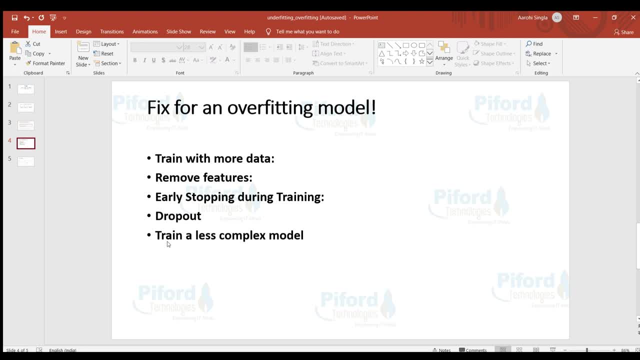 suppose data is very simple, right, the data set on which you are working is very simple, but the model which you are applying on it, the algorithm which you are applying on it, is very, you know, complex, and if you have lots of maths in it, that model is very complex. so what will happen on simpler data? 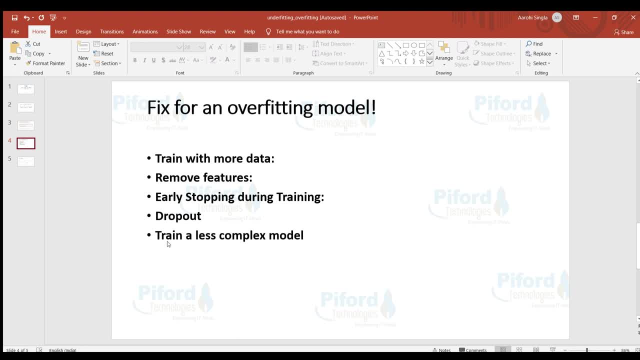 if you use a very complex method to solve that, so that is also be a problem of overfitting. so what you can do is you can try to train your algorithm with the less complex model. so these are the reasons like and the. these are the few ways by which you can, you know, reduce the problem of 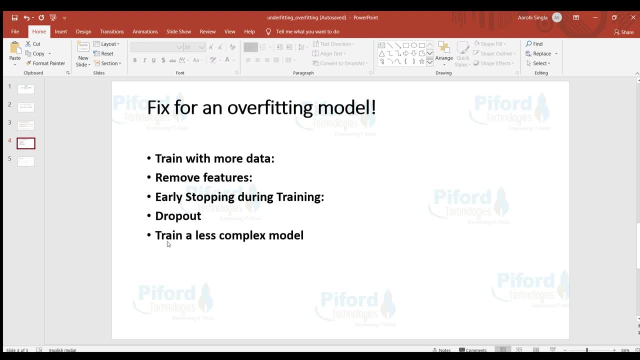 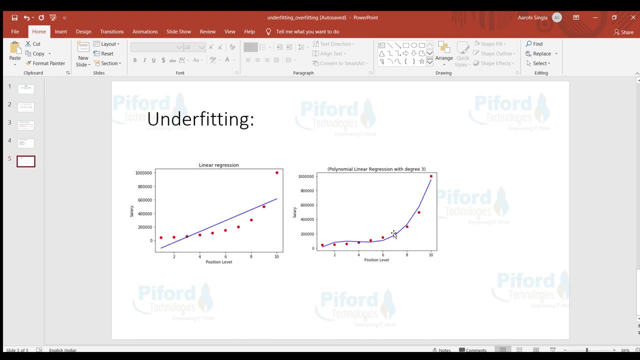 overfitting in simple terms, but don't worry, i'll show the practical example on it in today's class only. let me finish the theory first. okay, so we have studied overfitting, what is overfitting and how we can fix overfitting problem. now let's talk about underfitting. so, underfitting, so for. 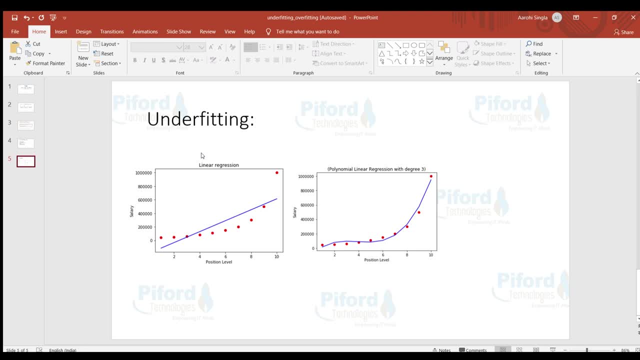 underfitting. let's look at this picture. so underfitting, i have already told you, means when model is performing poor on training data. so this is the first example. just check this example. see salary. So these red points are the actual data points. this blue line is the predicted result of. 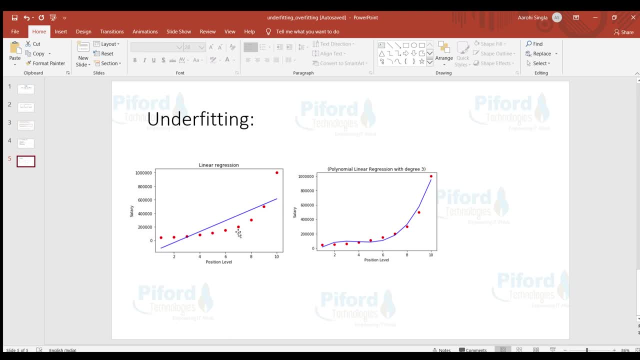 our algorithm. So over here, our algorithm is performing poor on the training data, because this is our actual data and this is how training results look like. So this is called, you know, underfitting problem. Even same example I have shown in my polynomial regression video also. 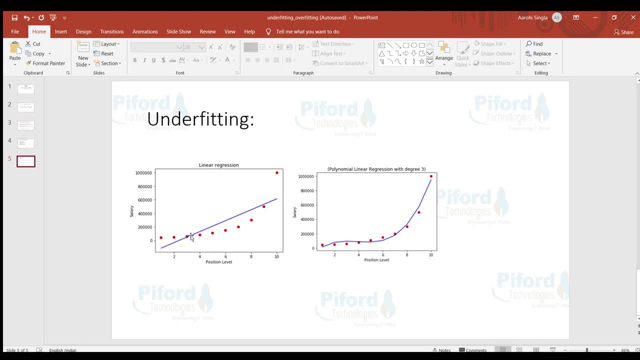 So this is the problem of underfitting. where actual data is like this and prediction is like this, means the algorithm which we are using here is not able to learn the data. and how we can solve the underfitting problem, and what are the different ways by which we can solve underfitting? See 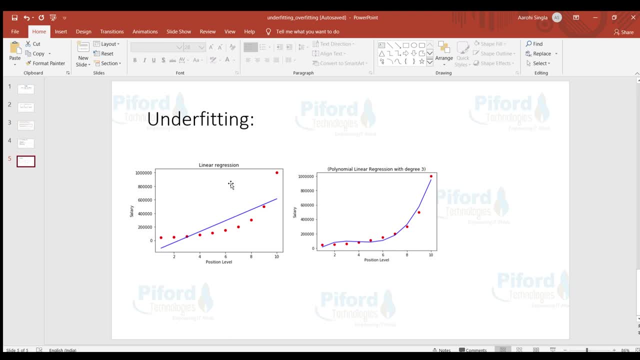 model is underfitting the training data when model perform poor on training data right. So this is because the model is unable to find the relation between x and y. Why this underfitting happens When? because the algorithm which we are applying on our data, that algorithm is unable to find the 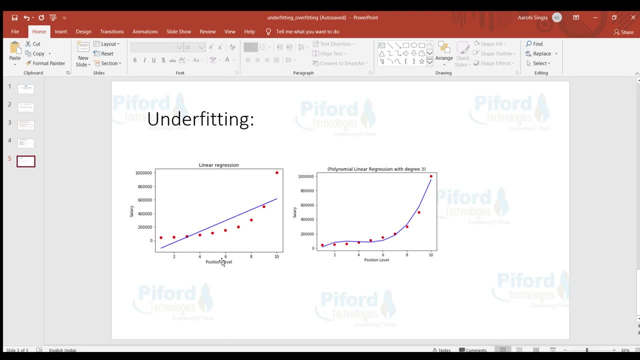 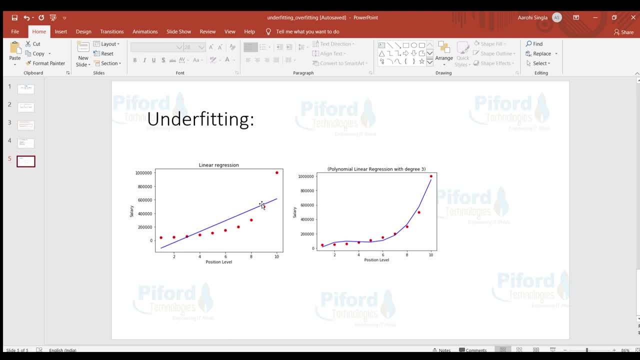 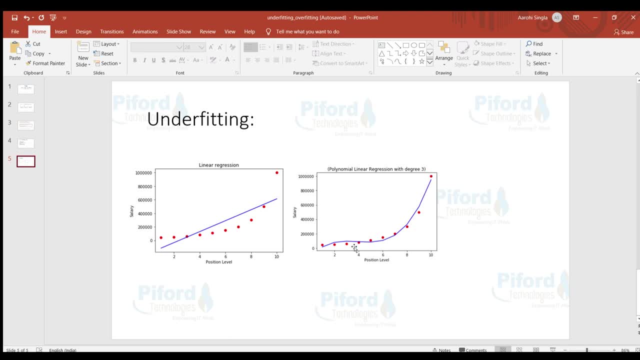 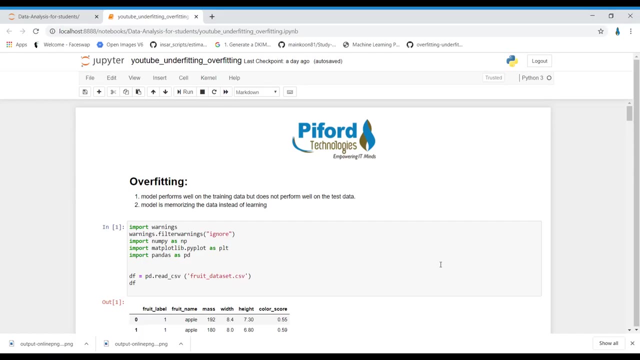 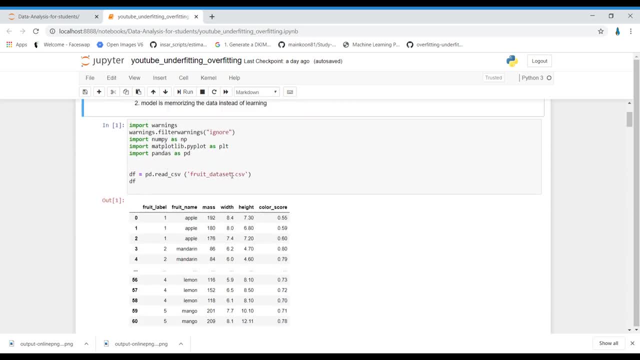 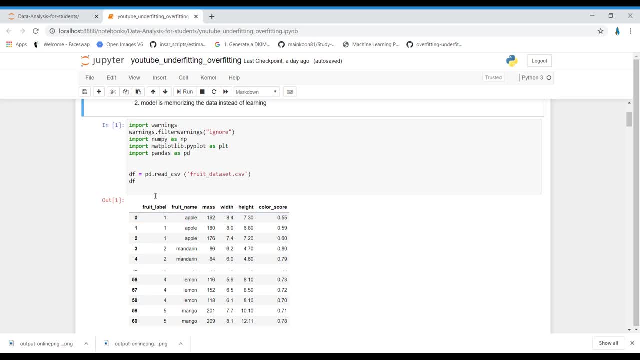 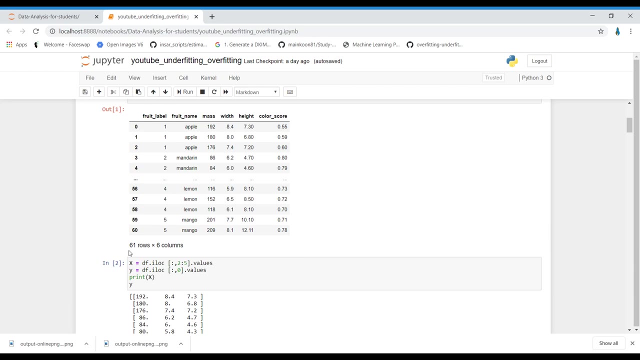 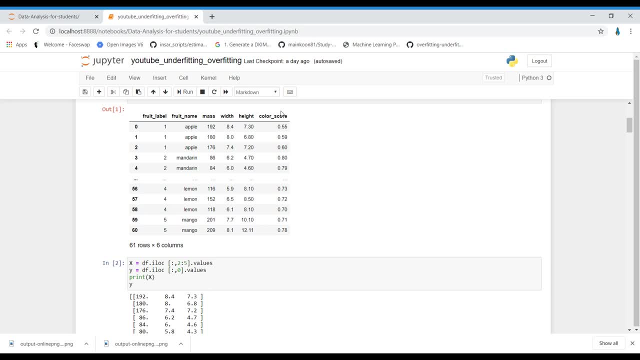 x and over here. i'm not using color score column on the basis of mass width and height. i want to predict the color label right, so i'm not using color score over here. so i've divided my data into x and y. after dividing the data into x and y. see, these are the three columns in x now and 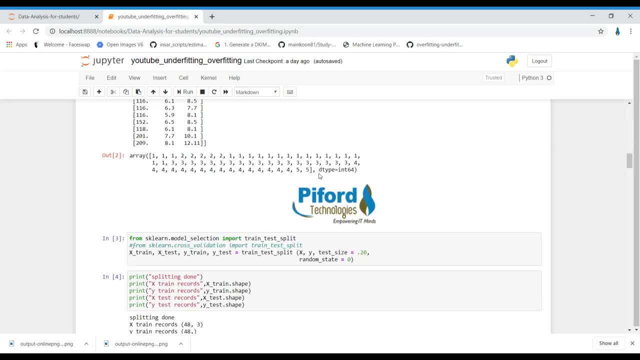 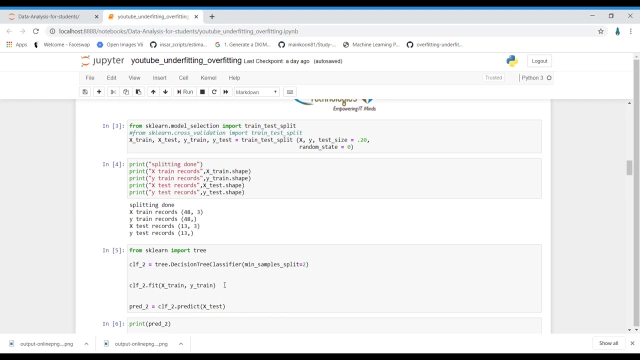 these are the different values in y now. now divide your data into train and test. so i've divided my data into train and test split. so these are the number of records: 48 records were there in train data and 13 records were there in test data. so now i'm applying the season tree. 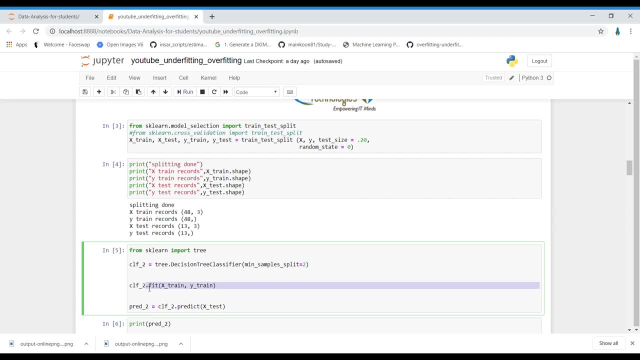 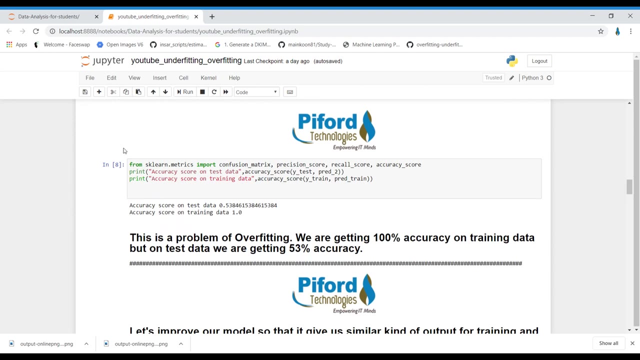 classifier on it. so first of all, i'm fitting data in it. by using dot fit, i'm training my algorithm. and then, by using dot predict, i'm predicting the results. so once we predicted the results, let's calculate the accuracy. see over here, if you'll see i'm calculating. 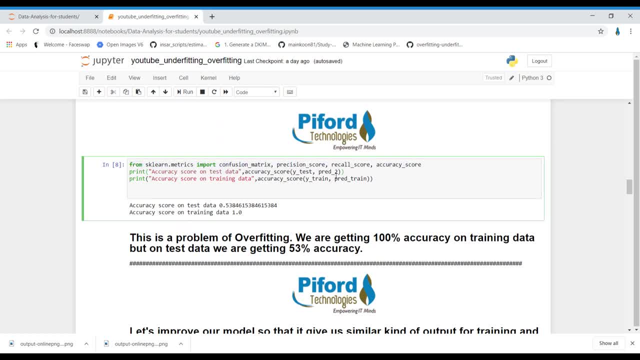 the accuracy. First of all, see what is accuracy? Accuracy simply means the difference between the actual Y value and the predicted Y value, And in Y test we have actual Y values of data and predict. underscore 2 is a variable in which we have, you know, predictions which we have made. 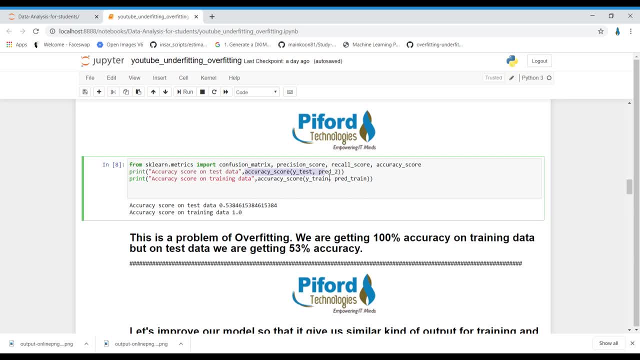 on X test data, So we will apply accuracy score on it. So what is the accuracy? we are getting 53% accuracy. we were getting on test data. In the same way, I am calculating accuracy for Y train and predict train. Y train is the actual data, which isn't, you know, which we have in a 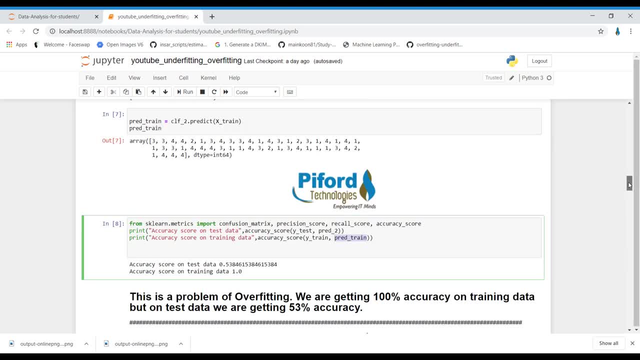 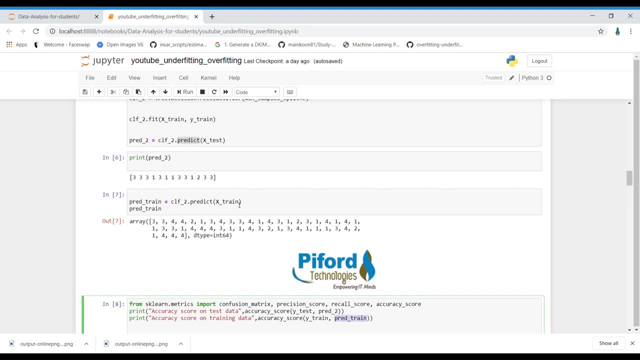 data set and this predict train I have calculated above. See over here. predict train: See. if you want to know the accuracy on training data, then we need to do make predictions for X train also. So we are getting 53% accuracy. We were getting 53% accuracy on test data In the same way. 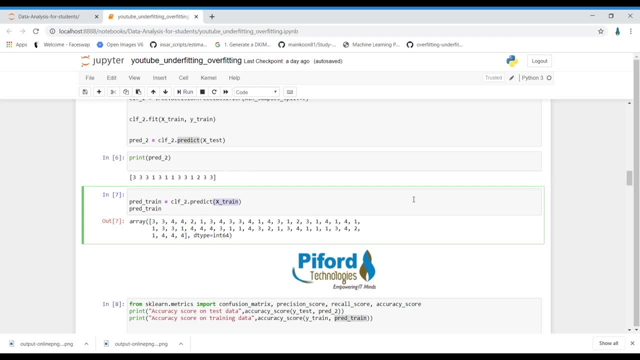 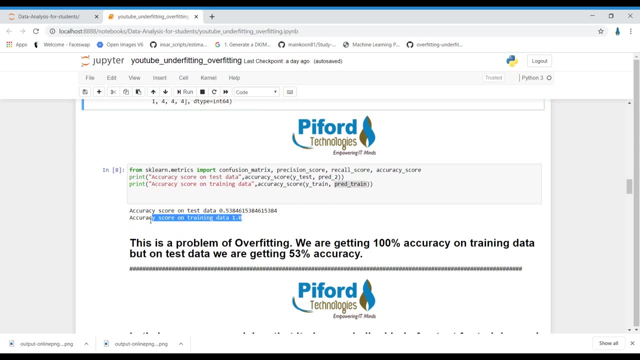 so I have made predictions on X train and I have made predictions on X test. Now, when I have calculated the accuracy, so we were getting this output: Accuracy score on training data is 100%, but accuracy score on test data is 53%, So that means this is a problem of overfitting. 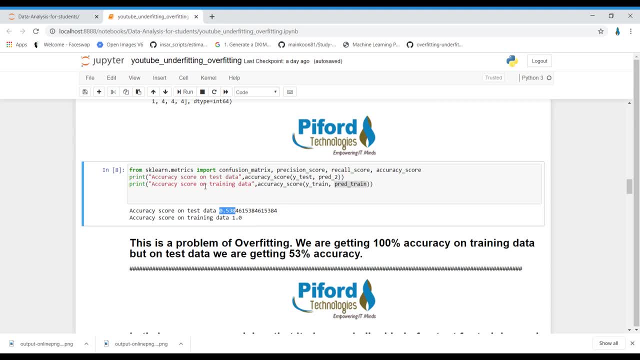 Now our task is to handle this problem of overfitting And, as I have told you in the previous video, if we can solve the problem of overfitting, we can either increase the data, right, So let's increase the data. So, before increasing the data, I just want to know like. 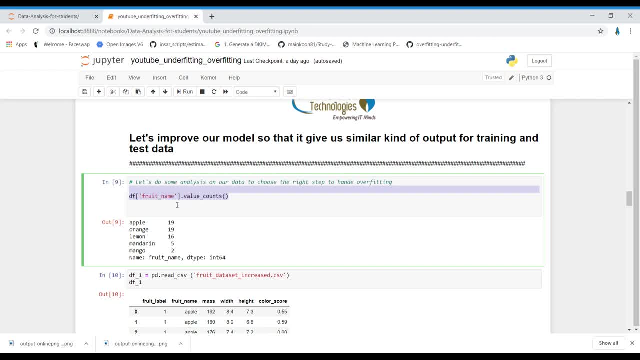 see, I have applied this value count on fruit name. I am doing some analysis on my data so that I can decide the right step. to, you know, solve the problem of overfitting means. rather, I need to increase the data, or should I use more, you know. 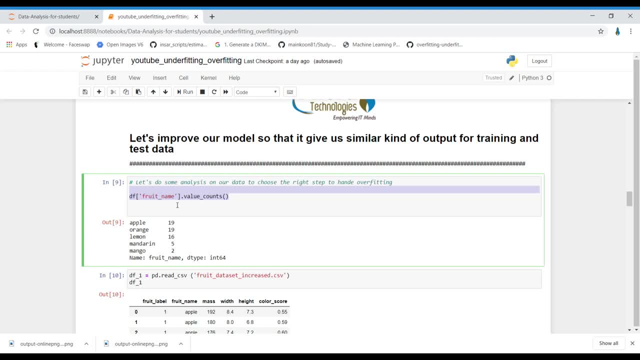 complex model or the simple model. So we have to decide the step to perform right. So for that I am doing data analysis on my this particular data set. So when I, on fruit name, I have performed value count, So from this these are the values which I get. So 19 records were belong. 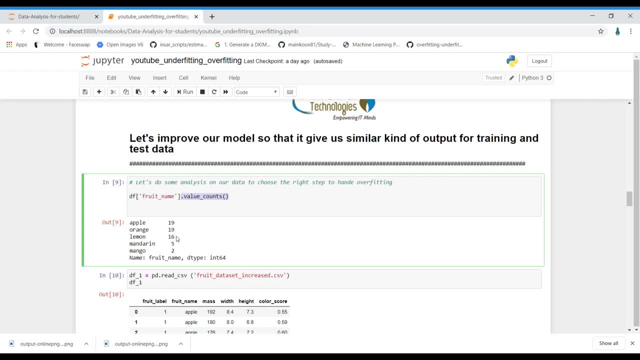 to apple, 19 records were orange and 16 records belongs to lemon. But for mandarin we have five records and for mango we have two records. These two means the data for these two classes is very less. So this is the problem of overfitting in. 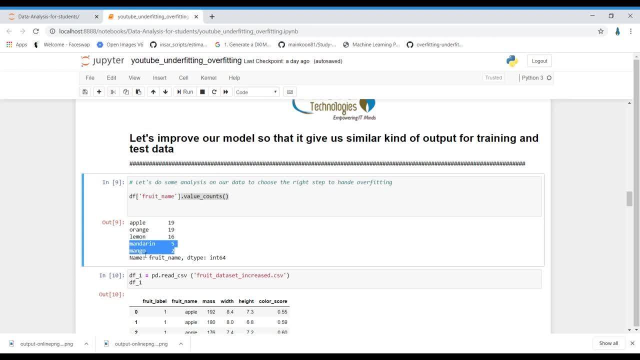 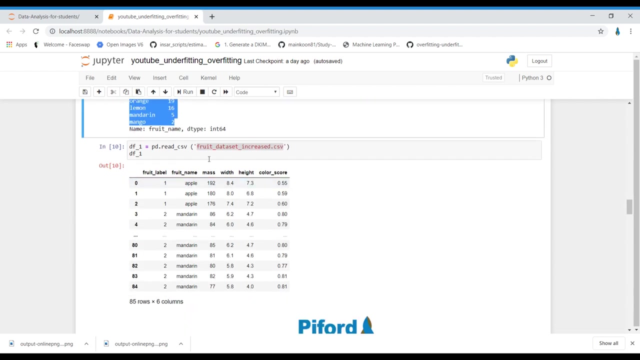 our case Now, what we can do. We need to increase the data for mango and we need to increase the data for mandarin right. So this is the file: fruit data increasecsv. So this is my csv file where I have manually inserted few records for mango and mandarin right. So now- and I am 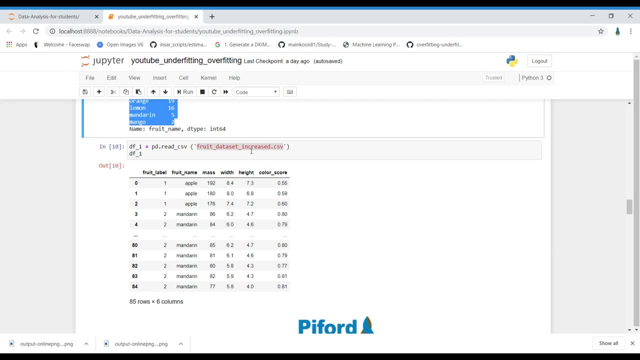 storing that in df underscore. one See, remember what I have done is earlier I was only having five records for mandarin and two records for mango, and we know like these two records are very less for these two classes, So that's why there is a problem of overfitting. So what I am, 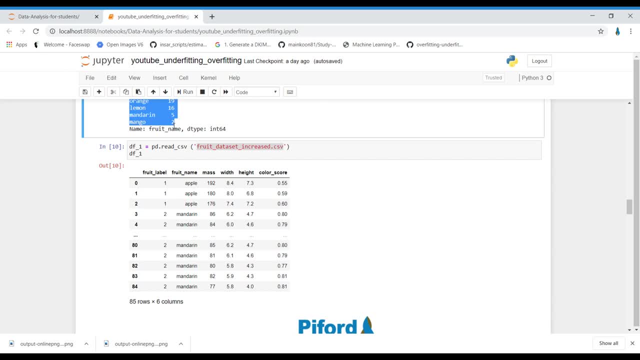 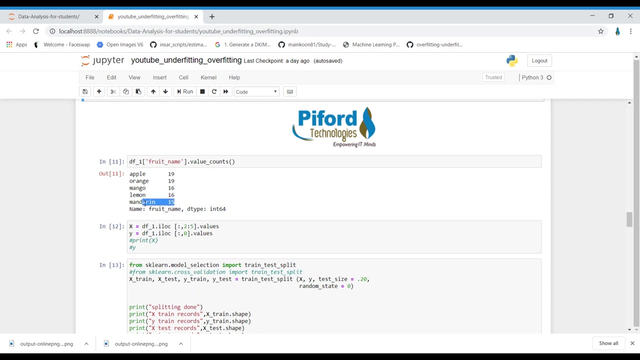 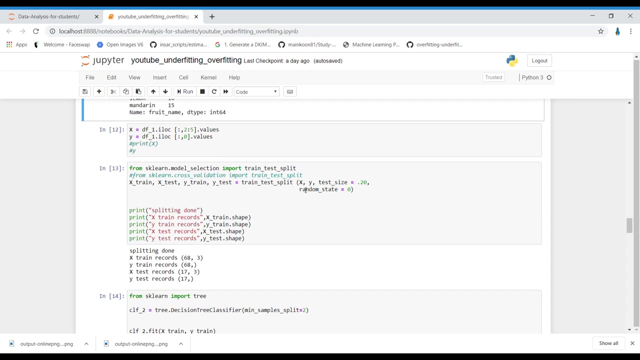 doing is I am manually opening my csv file and increasing the records manually for these two records, okay, These two classes So, and I have stored that result in this. Now we have again divided our data into x and y. right After that, divide your data for train and test split. 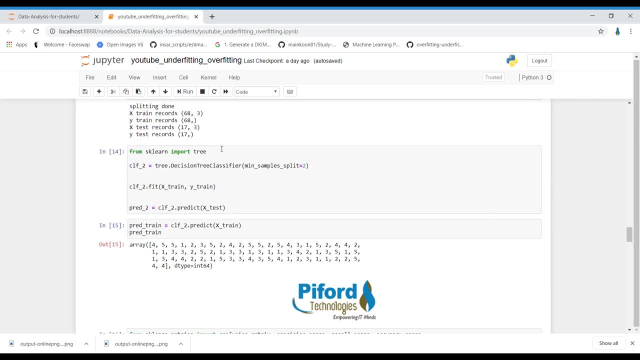 and then again apply the result. So now we have 15 records for mandarin and for mango. So we have 15 records for mandarin and for mango. So now we have 15 records for mandarin and for. 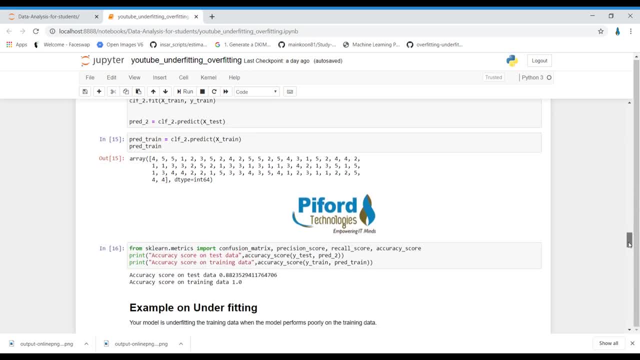 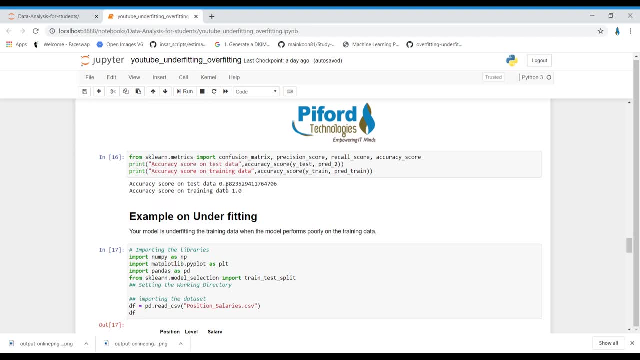 season tree on it. and then we are checking accuracy again. So over here you will see, accuracy on test data is 88%, Previously it was 53% but now it is 88%, and accuracy score on training data is 100%. So over here we have improved the result. So over here we can say: 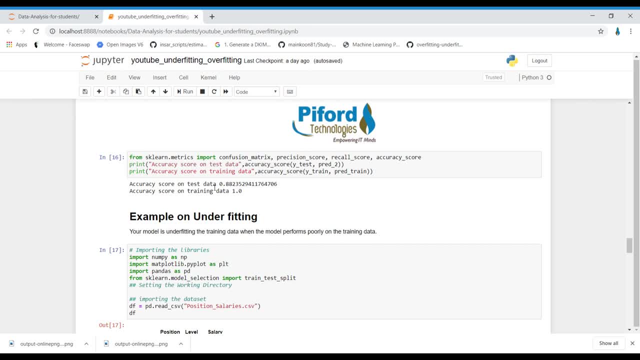 that the problem of overfitting. we have worked on it and the result is good. So over here results were improved. but if you want to improve your results more, then you can more increase your data. But over here our problem is somehow solved. Previously we were getting how much. 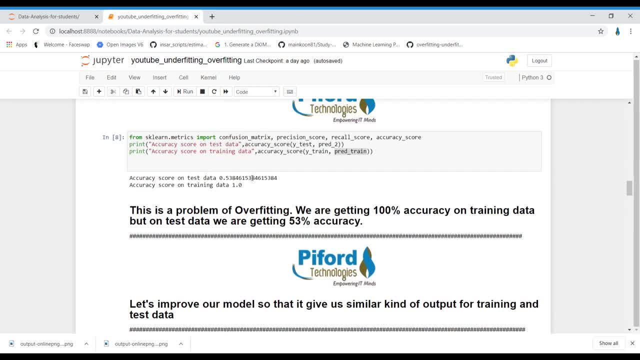 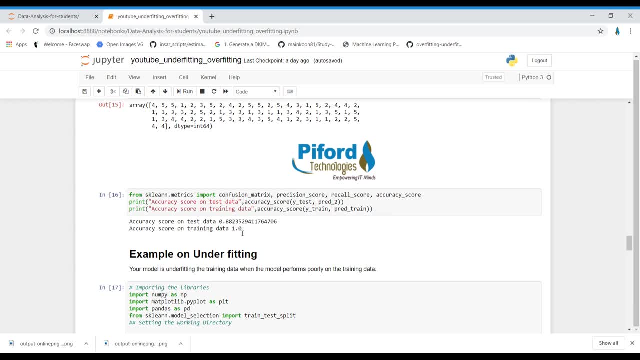 accuracy we were getting on previous data- 53% right, But now our results are somehow closer to the output: 88% accuracy we are getting on test data and 100% accuracy we are getting on training data. So this is how I have solved the problem of overfitting right Now. 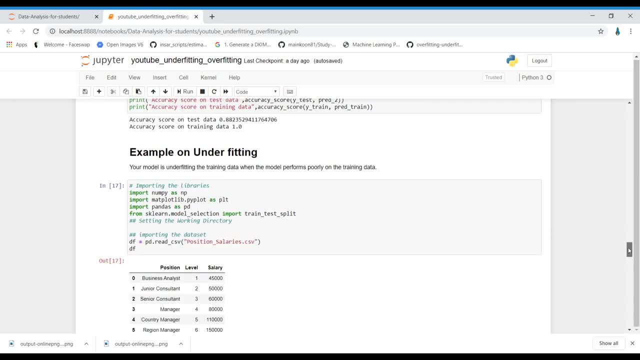 let's discuss about underfitting. For underfitting, I will be using the same example which I have used in polynomial regression. That is a very good example, right? So underfitting simply means when your model is performing poorly on the training data itself. And what is the reason? 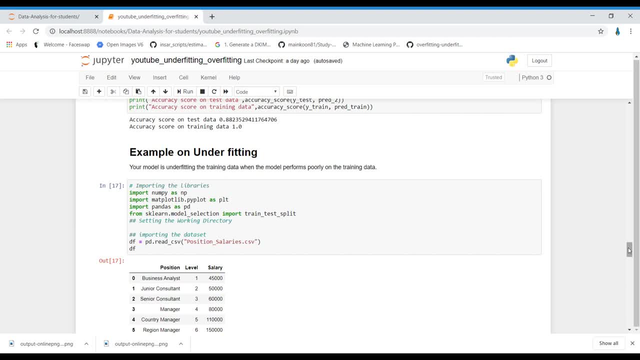 for it. The reason for it was the reason for underfitting- is that the model- maybe the model which you are using- is too simple For the data and that model is not able to understand the data. and if we want to solve the underfitting problem, then we need to change our algorithm to a complex model, right? So 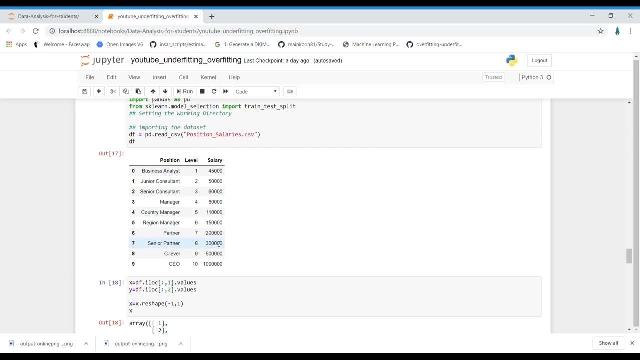 this is the data position salariescsv file. right On this data I am working. So level column is the label encoded form of position column only. So in x we have level column and in y we have salary column. So I have divided my data into x and y over here. 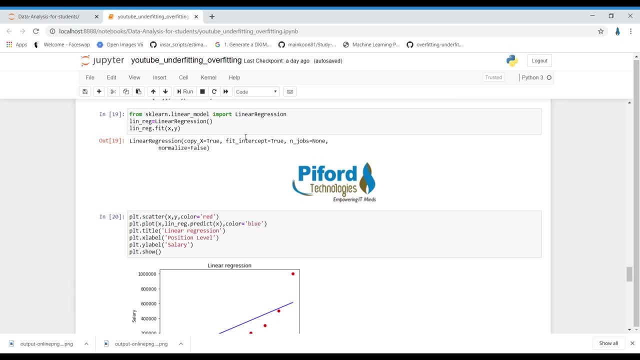 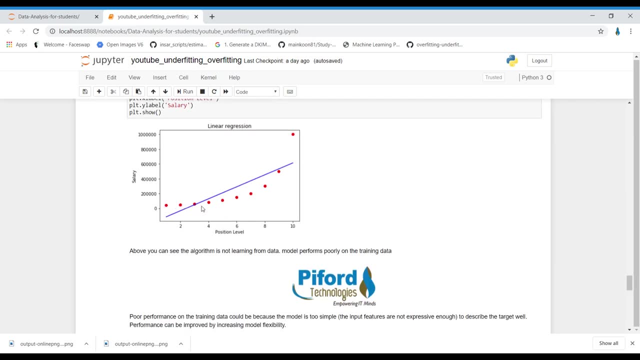 So thiseninazi. so after dividing my data into x and y, are performing linear regression on that data. So when I perform linear regression on that data, so this kind of output I am getting. So red dots are the actual data points and blue line is the predicted result. 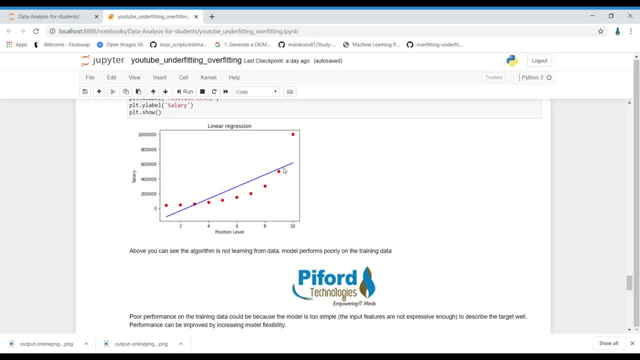 So over here we can see clearly that model is performing poorly on the training data. Model is not able to learn this data. Why? Because the model which we are using here is too simple and we need to over fill the data so that our model is able to at least. Нам, in that case, is able enough to find free sv. So before that model is actually set to 1 critical data. So at this stagevens C, Let's think about the models. we can start and we will look at the other models. These two models are quite similar to each other. Cause the model. 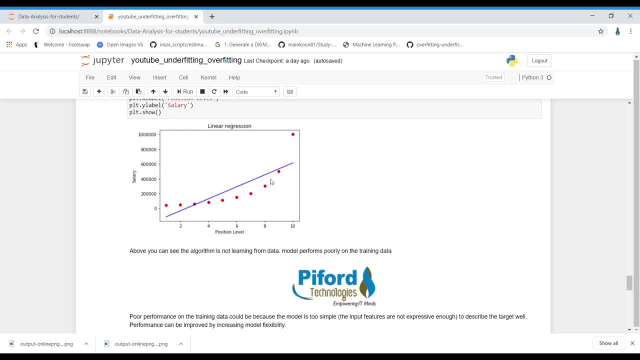 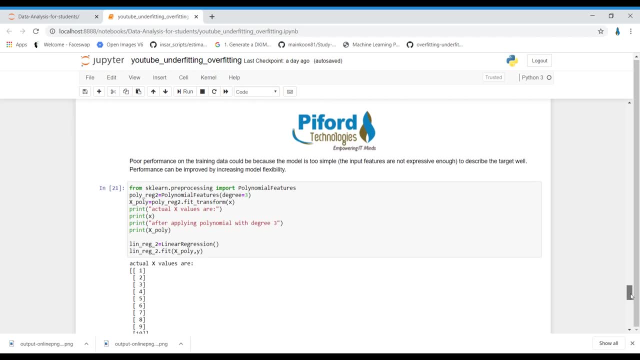 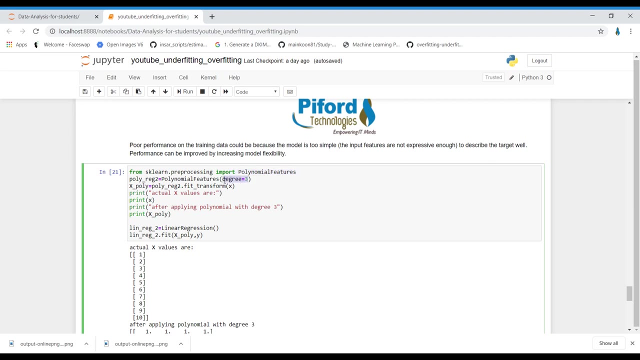 too simple for the data. The model which we are using is linear regression and the data is non-linear, So let's choose the more complex model. The more complex model which I am using over here is polynomial feature and I am changing my x with degree 3, right? So see the concept.